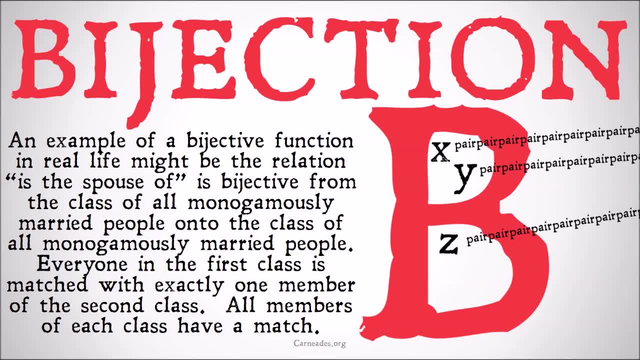 Everyone in the first class is matched with exactly one and only one member of the second class, and all members of the second class are matched with exactly one and only one member of the first class. All members of each class have exactly one and only one match. The relation. 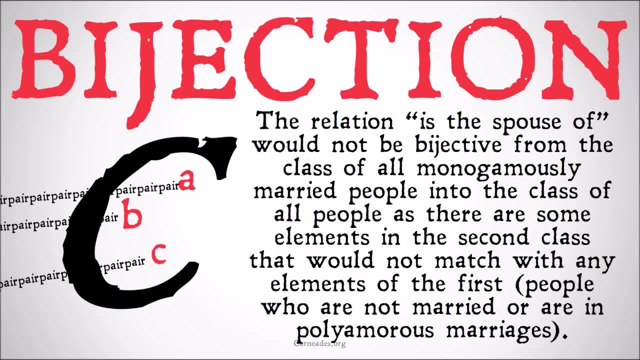 is the spouse of would not be bijective from the class of all monogamously married people into the class of all people. As, for a couple of reasons, As there are some bijective functions, some elements in the second class which would not match with any elements in the first people. 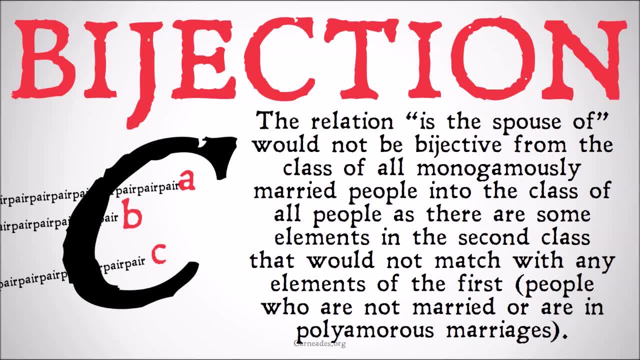 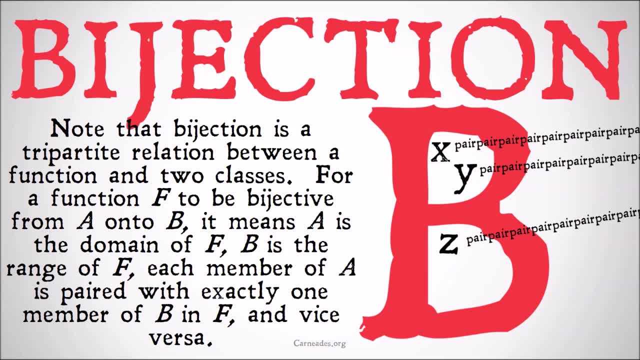 who are not married at all or people who are in polygamous marriages. Note that bijection is a tripartite relation between a function and two classes. For a function, f, to be bijective from a on to b, it means that a is the domain of f, b is the range of f and each member. 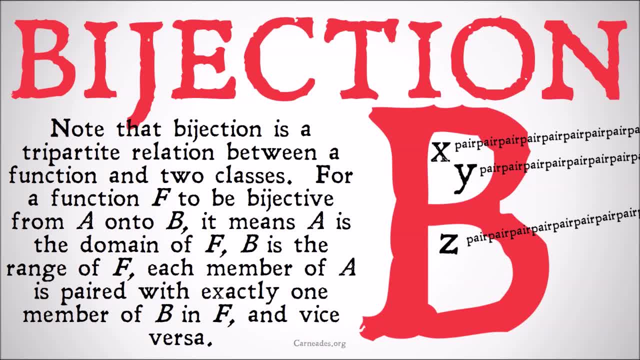 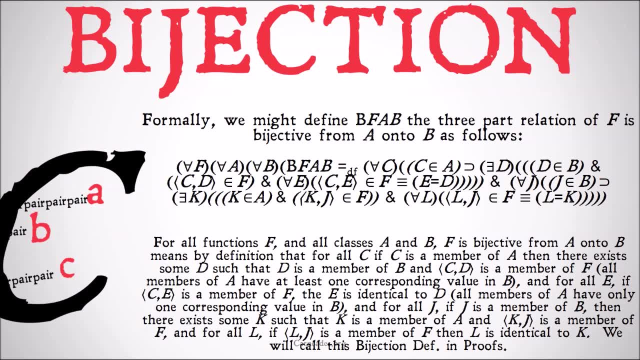 of a is paired with a. Formally we might define b, f, a, b. the tripartite relation of f is bijective from a on to b as follows: For all functions, f, in all classes, a and b. f is bijective from. 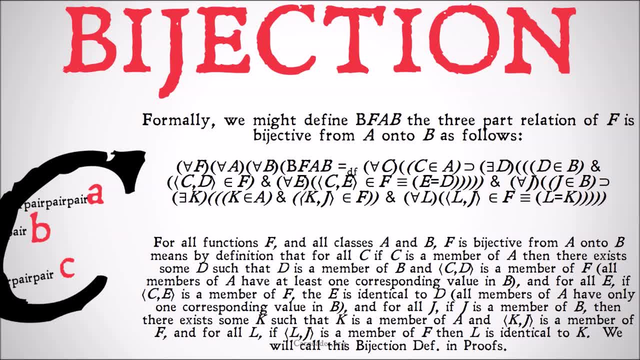